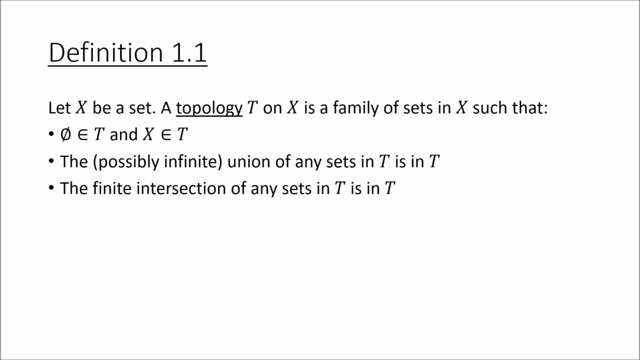 and the finite intersection of any sets in T is in T Theorem 1.2.. A subset Q of the real numbers is open in the Euclidean topology if, and only if, it is a union of open intervals. And we can see the definition of the Euclidean topology here: Proof. 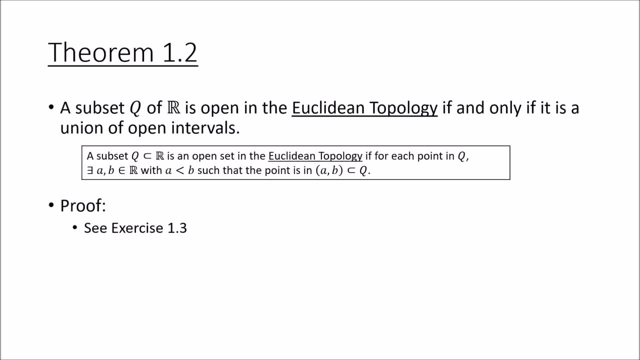 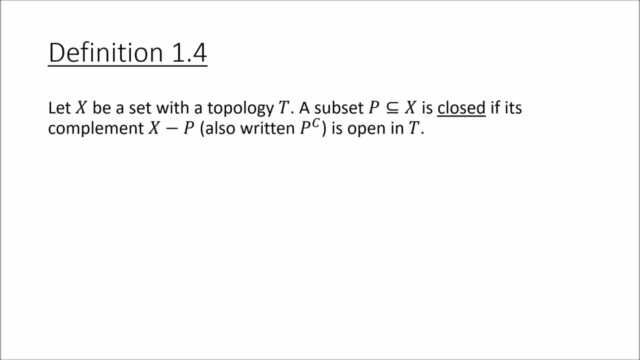 For the proof: see exercise 1.3.. Exercise 1.3.. Proof theorem 1.2.. Definition 1.4.. Let X be a set with a topology T. A subset P of X is closed if its complement. 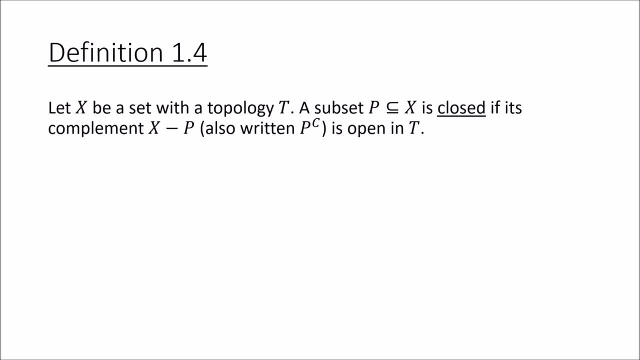 X minus P, also written P. superscript C is open in T Definition 1.5.. The closure P bar of a set P is the union of P and all its limit points. where a limit point is closed, if it is a union of P and all its limit points. 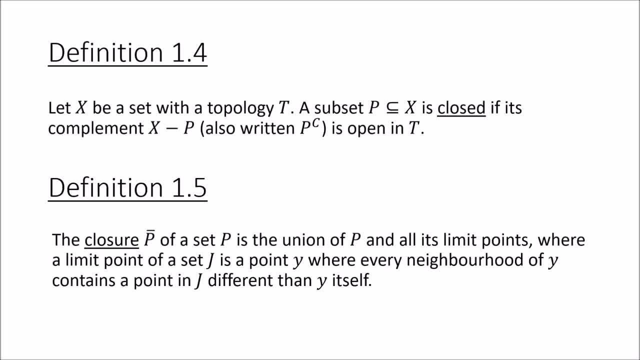 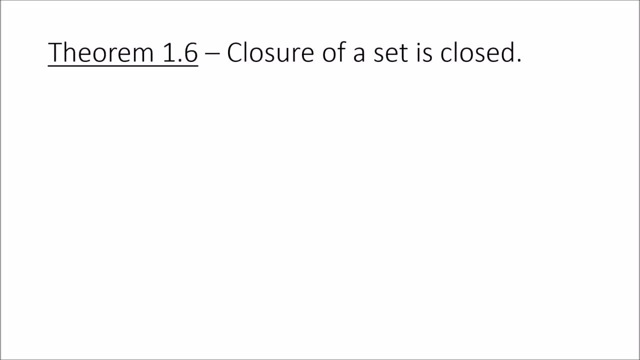 Definition 1.5.. The closure P bar of a set. P is the union of P and all its limit points. where a limit point of a set J is a point Y, where every neighborhood of Y contains a point in J different than Y itself. Theorem 1.6.. The closure of a set is closed. 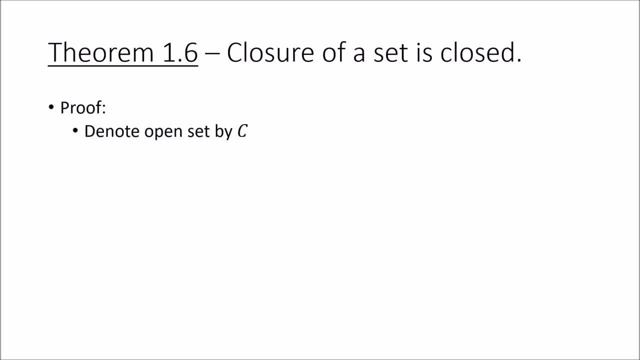 Proof For this proof. we'll denote open sets by the letter C, we'll denote ordinary sets by the letter P and we'll denote points by the Greek letter capital, Rho. Suppose that Rho is not in P bar, Then there exists a C? Rho, such that Rho is in C Rho and C Rho. 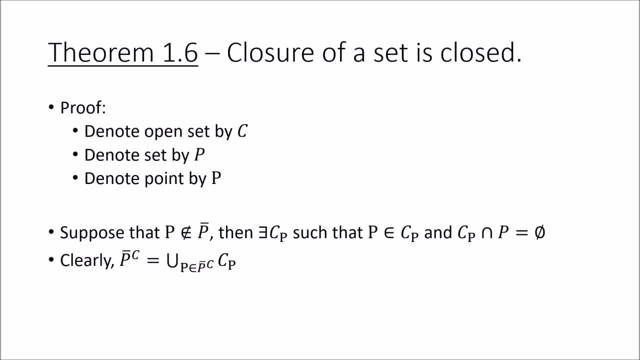 intersect P as the empty set. Clearly, P bar C is the union of sets C- Rho, such that Rho is in P bar C. Since the union of open sets is an open set, this must mean that P bar C is open. Therefore. 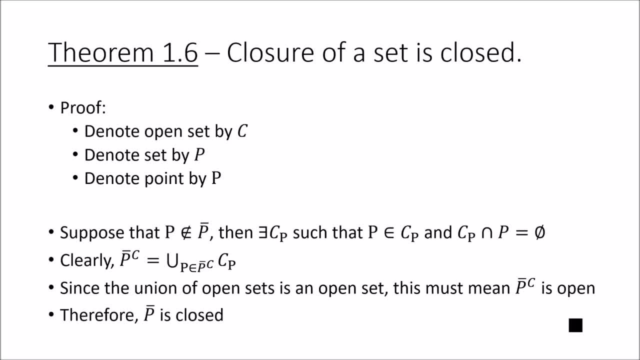 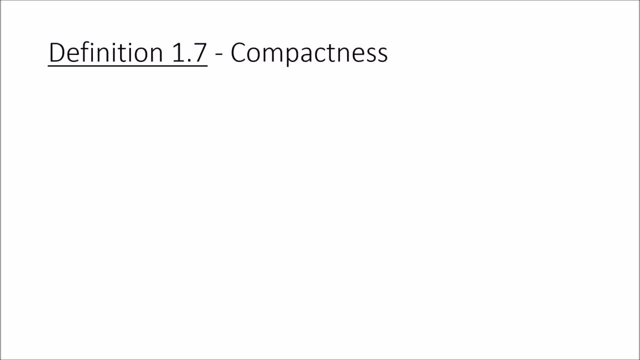 P bar is closed. This completes the proof. If you find this proof confusing, please look at this easy-to-understand diagram. Definition 1.7. Compactness. Now I'd like to emphasize that this definition is very, very important. It's a very, very important definition. It's a very 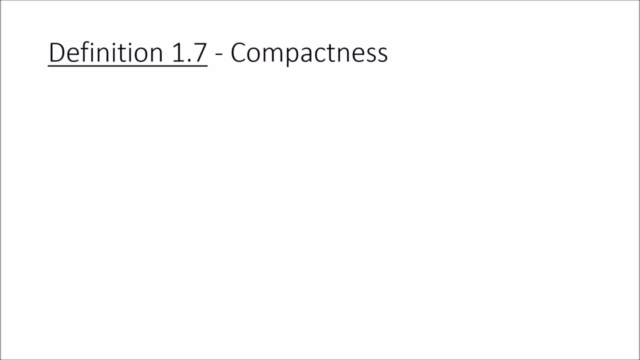 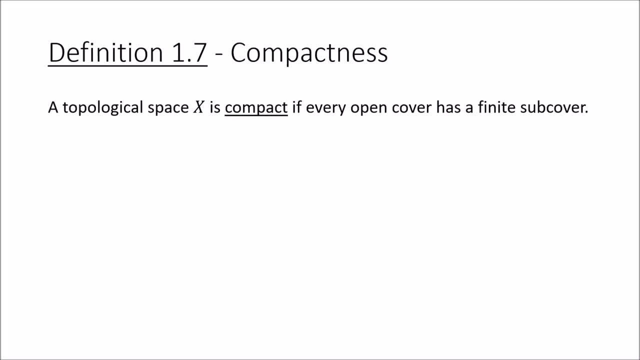 X is compact if every open cover has a finite subcover. So please make sure you understand this definition. Theorem 1.8.. The Heine-Berl theorem. The Heine-Berl theorem states that every closed-bounded subset of Rn is compact Proof. Start by taking a closed-bounded subset, P.